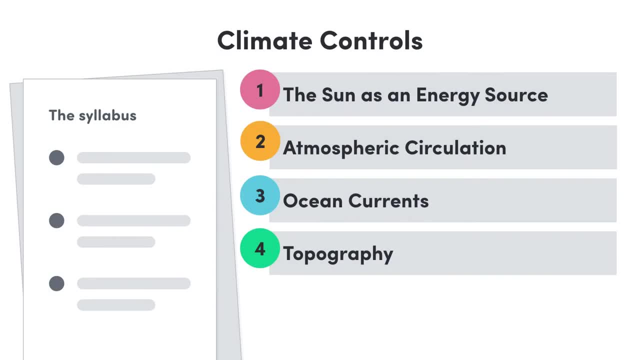 Hi there and welcome back to Atomy Geography. This lesson is the second part of our two-part series on the global climate. Last time we introduced climate and the characteristics of different climate zones. This time we're taking a look at the factors that affect and. 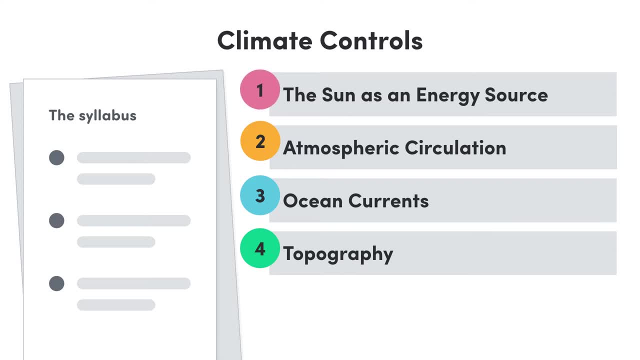 control the global climate. First we'll have a look at the sun as the main energy source driving climate factors, and then we'll tackle the factors themselves: Atmospheric circulation, ocean currents and topography. So let's start by considering the driving force behind all of 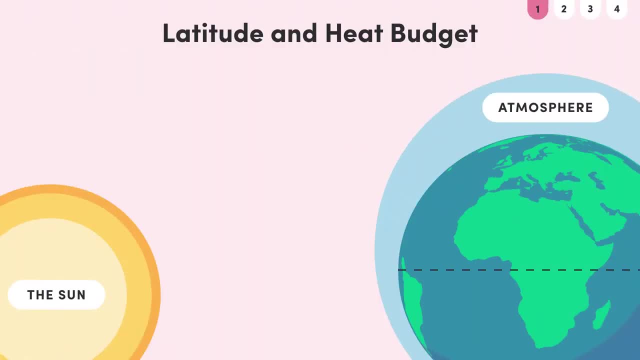 these climate processes. The sun, Solar energy that reaches the earth is called insulation. Once solar radiation reaches the earth, it can either be reflected back into space by clouds or dust, or it can be absorbed by the atmosphere or the surface of the earth. Insulation can also be. 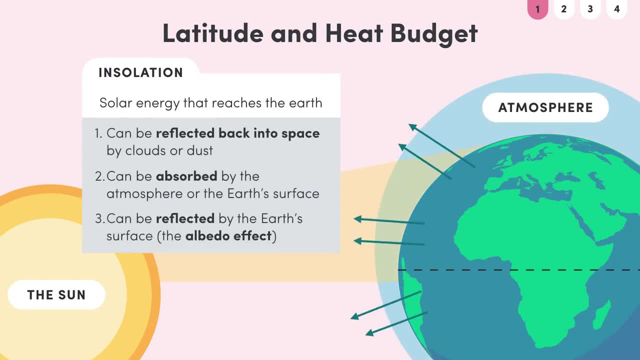 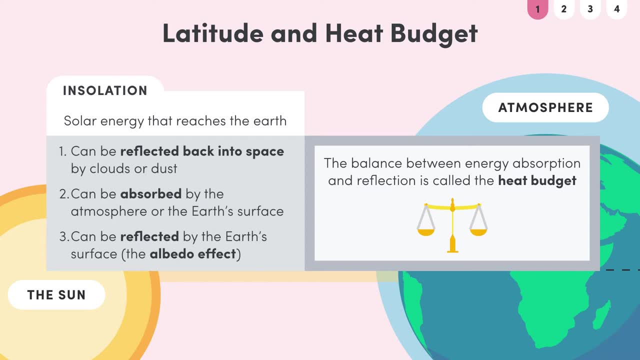 reflected by the surface of the earth, which is called the albedo effect. The balance between absorption and reflection of solar energy is called the albedo effect, The balance between the heat budget of the earth, So the temperature difference between the equatorial and polar. 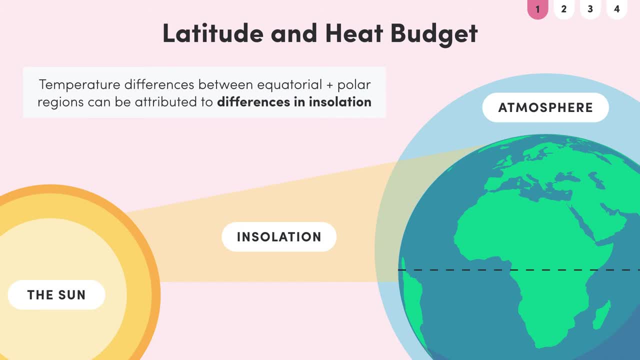 regions can be attributed to the difference in insulation at these regions. As you can see in this diagram, the equatorial area of the earth faces the sun directly, meaning insulation is much more concentrated over a small area, leading to more energy at the surface. It also doesn't 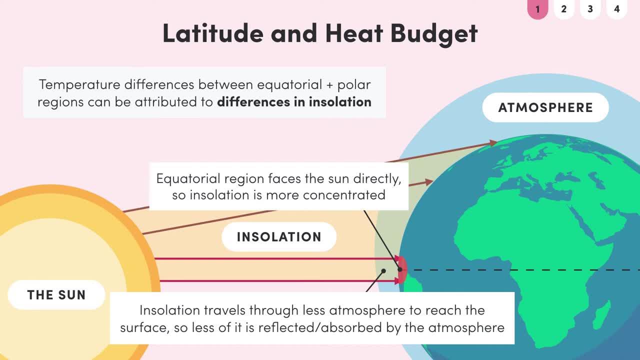 have to travel through as much atmosphere to reach the surface, so little insulation is reflected or absorbed by the atmosphere. This means that the surface temperatures are much more concentrated at the equator are high. In contrast, the poles never face the sun directly, meaning insulation can. 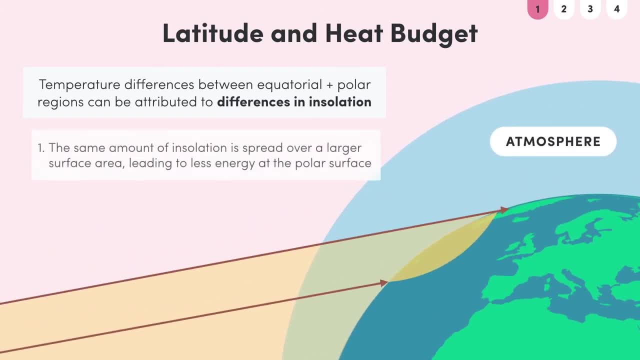 only reach the surface near the poles at an angle, So the same amount of insulation is spread over a larger portion of the polar surface when compared to the equator, leading to less energy at the surface. It also has to travel through more atmosphere, so is more likely to be absorbed or 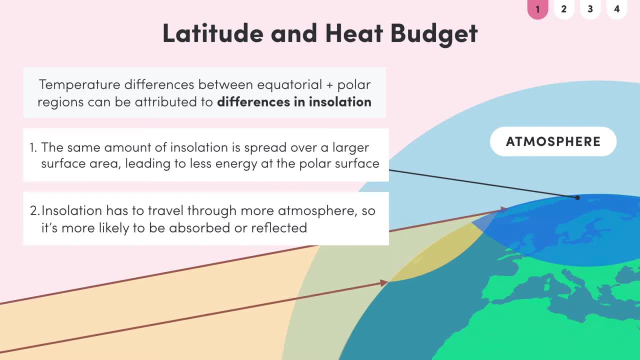 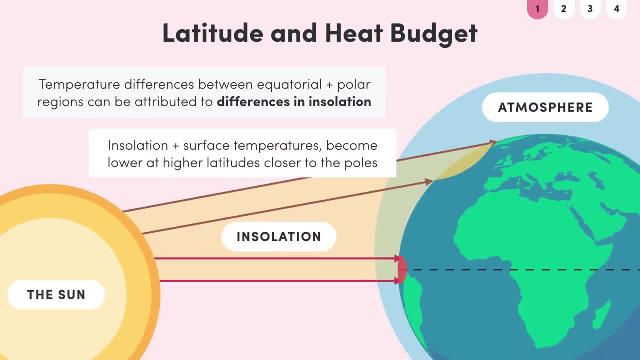 reflected. Finally, ice reflects more sunlight than water or earth, causing stronger albedo effects at the poles. A combination of all of this means that insulation, and therefore surface temperatures, become lower at higher latitudes closer to the poles. So now we understand how insulation creates different temperature zones. 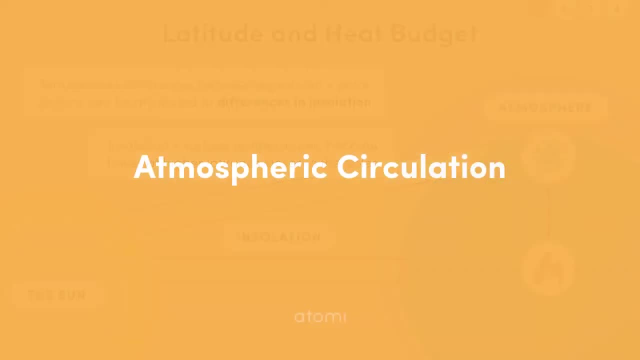 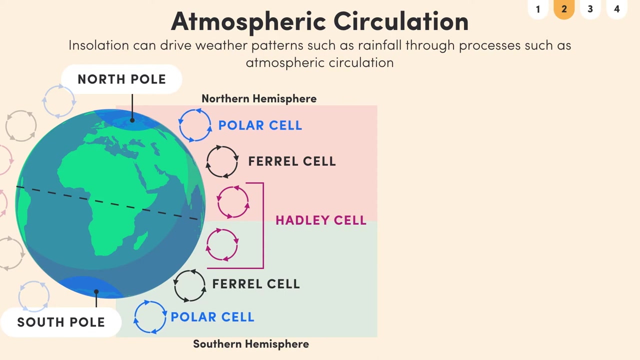 on earth. but how does it drive other weather patterns like rainfall? Well, let's start with atmospheric circulation, which occurs in a specific pattern. As you can see in this diagram, there are three cells of air circulation in each hemisphere. The key to these cells is air density. Essentially, all of the air that is in the atmosphere is air density. So if you look at the diagram, you can see that there are three cells of air circulation in each hemisphere. The key to these cells is air density. That is another type of air that is in the atmosphere, since there was heat generated topics: 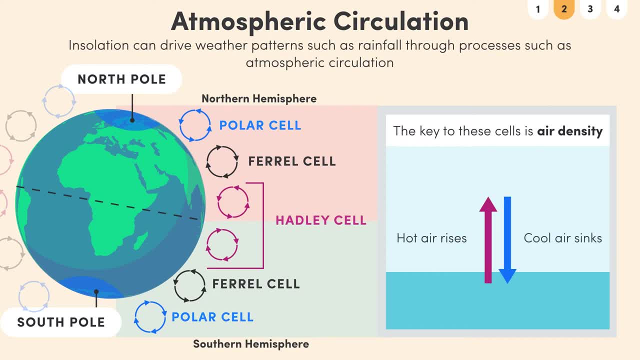 in the atmosphere at class area. so in fact here the temperature is constantly changing. Forest is less strong, so as this air to energy, air do not rotate, so much is less dense, so hot air rises and cold air sinks. As hot air rises, it creates low pressure zone. It also carries water vapor. 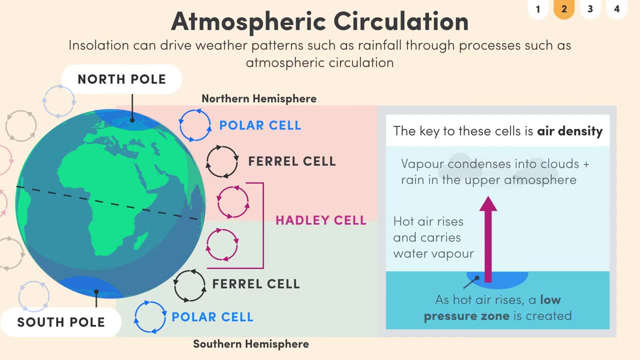 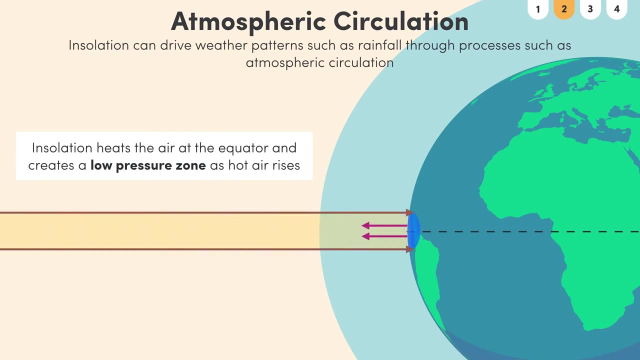 up with it, which then condenses in the upper atmosphere to form clouds and rain. In contrast, as cold air senses, it created a high pressure zone characterized by dry conditions. As we can see, insulation heats up the air at the equator and creates low pressure zones as the hot air rises. As this air rises its splits and gapgeh in the atmosphere. It is also filled with light heat. a spread between the east and south ocean enhances more heat generation through in vitro air mediums. and sounds in this video e local water temperature and nothing as那个 actually evening in front of every. 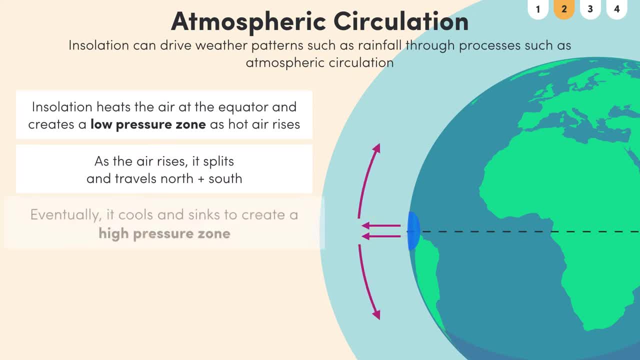 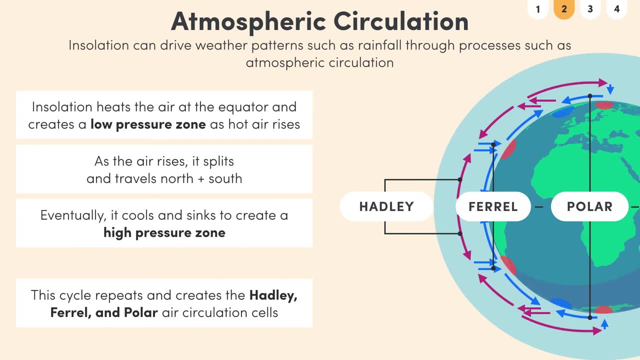 It splits and travels north and south, eventually cooling and sinking again to create a high pressure zone. This cycle repeats, creating three bands of rotating air called the Hadley, Ferrel and Polar cells. The circulation of these three cells creates alternating high and low pressure bands, which 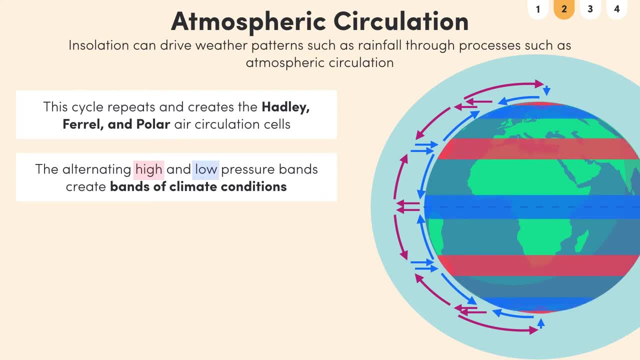 in turn create bands of climate conditions. Rainy conditions dominate where air rises at low pressure areas around the equator and 60 degrees latitude, while dry conditions dominate where the air sinks at the high pressure areas, at the poles and at 30 degrees latitude. 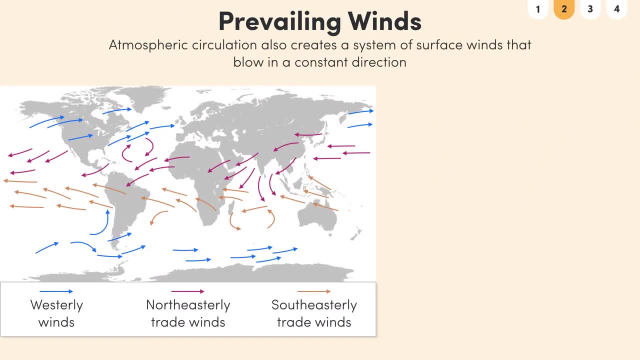 Furthermore, atmospheric circulation creates a system of surface winds that blow in a constant direction. These prevailing winds will form as air is sucked from high pressure areas to low pressure areas. Prevailing winds often play a role in determining regional climate. For example, if the prevailing wind blows inland from the ocean, the climate will be. 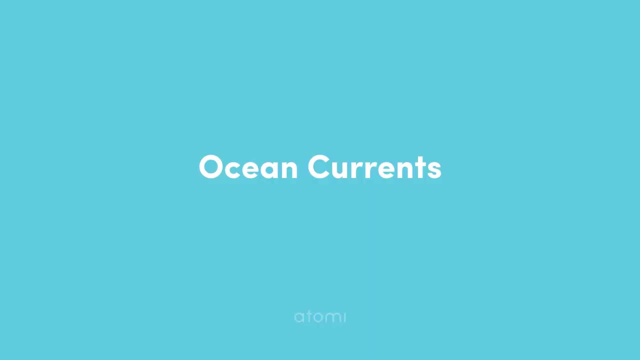 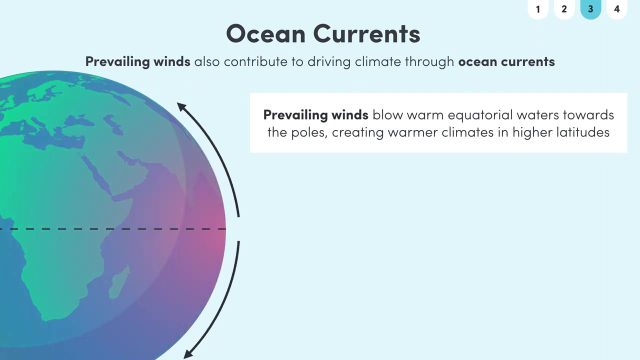 more rainy. Prevailing winds play another role in driving climate – ocean currents. Winds blow warm equatorial waters away from the equator to the poles, creating warmer climates in higher latitudes. This effect becomes weaker further away from the ocean, so that climates in regions far